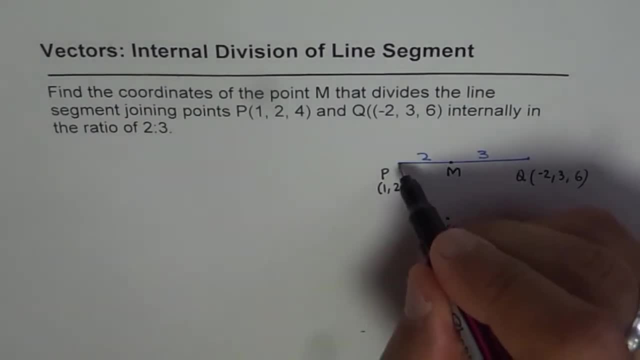 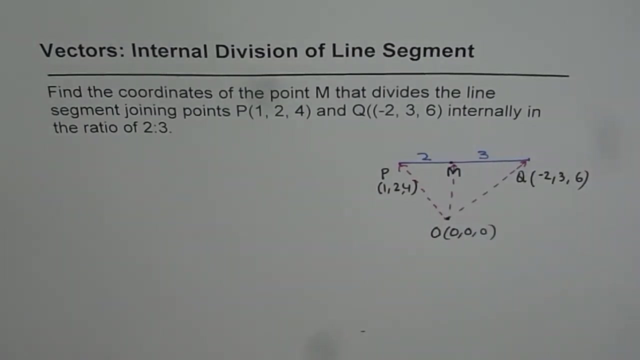 have position vectors OP, that is this position vector- OP and OQ, OM. So these are now my three position vectors and that will help us to solve the question. Now, what is OM equals to? So from the formulas which we have derived, we can say: OM is equal. 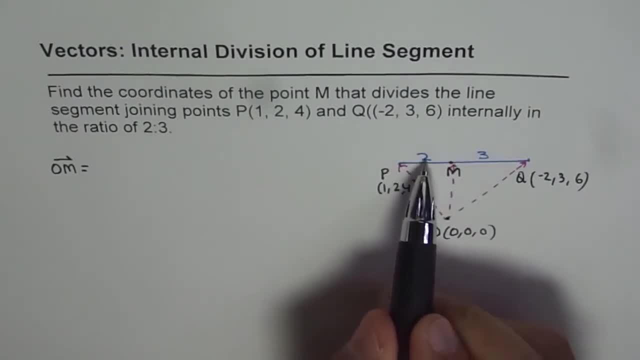 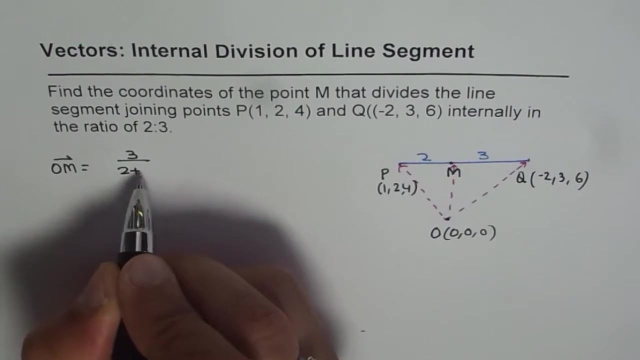 to this is: ratio of 2 is to 3.. So point P is 1, 2 and 4.. We have to multiply this by 3. So it is actually 3 over 2 plus 3 times OP, right. 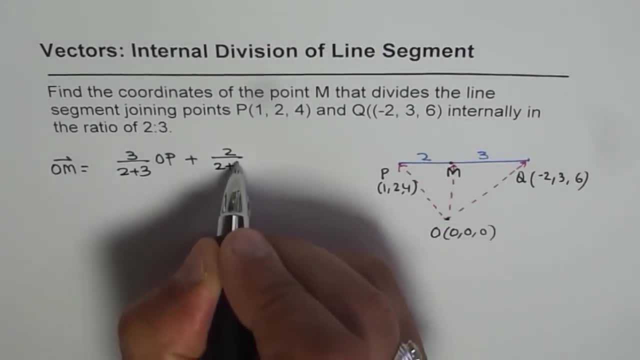 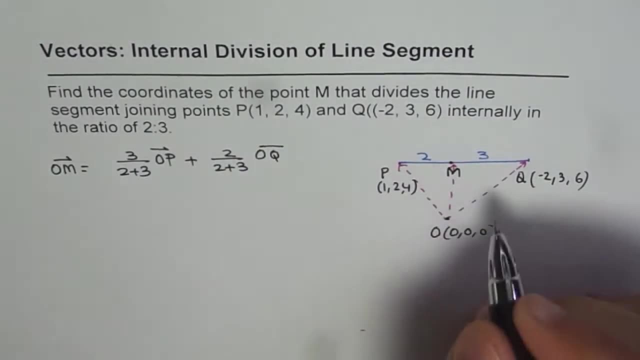 Yes, So 5 plus 1 over 3 plus 2 over 2 plus 3 times OQ. So that is how OM is related with OP and OQ, and this is the formula which we derived in previous videos, So we will just apply. 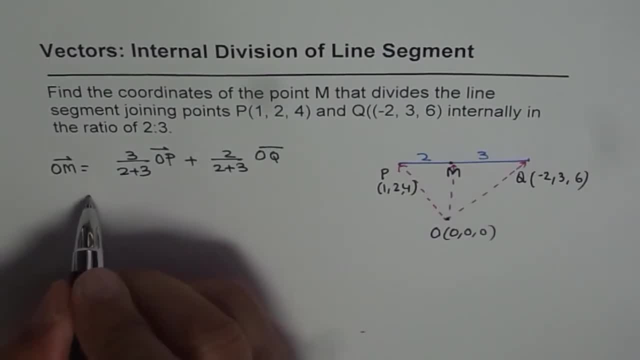 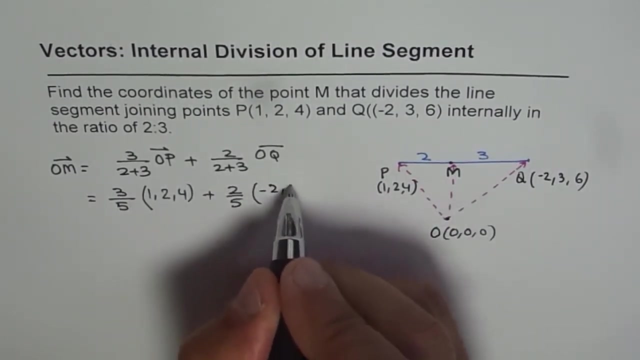 this and find out what is OM. So from here we get OM equals to 3 over 5.. OP is 1, 2, 4.. Okay, plus 2 over 5. OQ is minus 2, 3, 6. 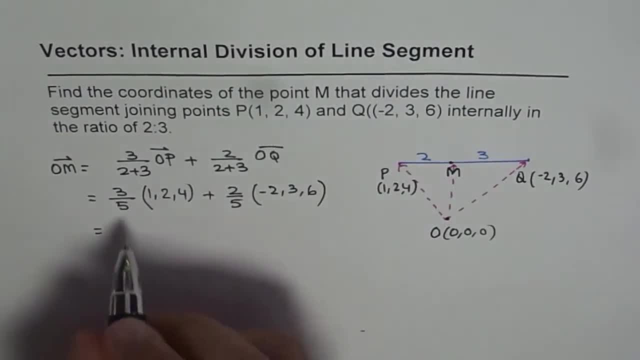 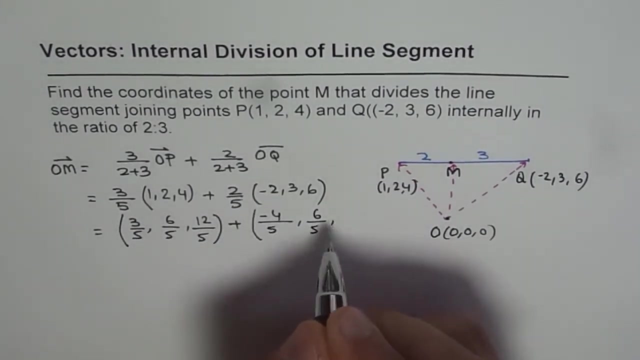 so let's solve it. we get 3 over 5, 6 over 5 and 12 over 5, plus minus 4 over 5, 6 over 5, 12 over 5. so when we add them, we get 3 minus 4 is minus 1. 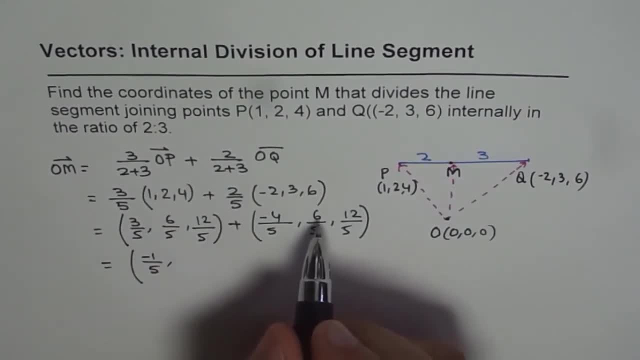 6 plus 6 is 12, so we get 12 over 5, and 12 plus 12 is 24. so these are the points. so that is how vector OQ, OM is defined. now, if OM is minus 1 over 5, 12 over 5.